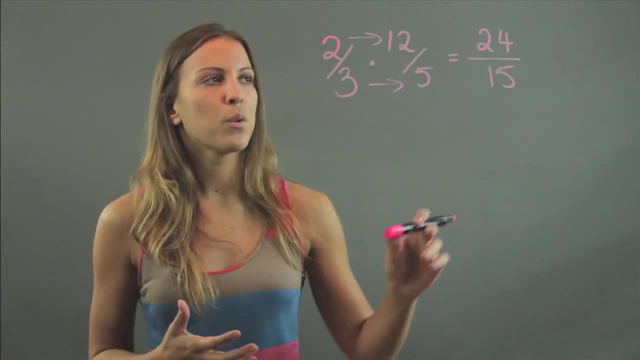 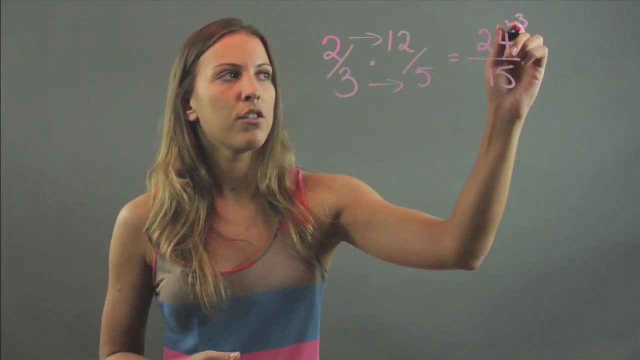 But almost always when dealing with fractions, you want to reduce when possible. So we're looking for a common factor of 24 and 15.. A number that can go into both 24 and 15 is 3.. So we're going to divide the numerator and denominator by 3, and when we do that we get 8 over 5.. 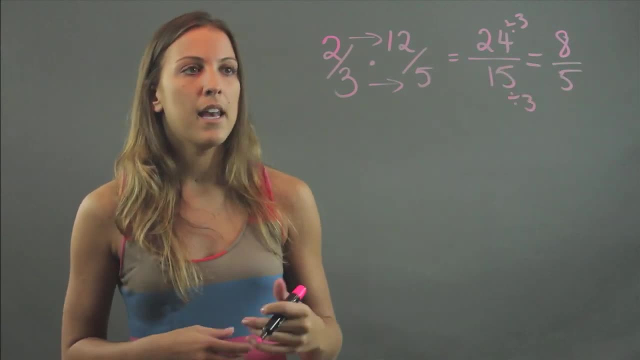 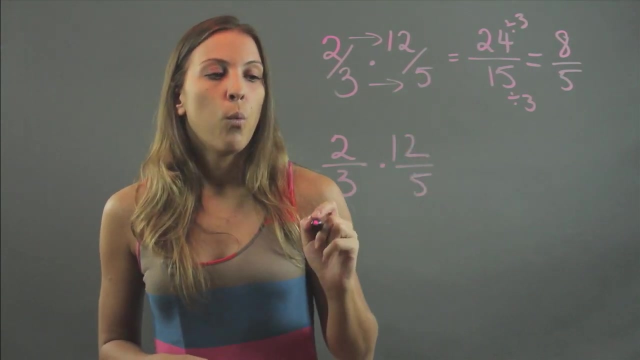 And we can't simplify any further. so that would be my simplified answer. Now, the other way, and the way that I would have multiplied this if I had this problem, is 2 thirds times 12 over 5.. What you do is you look to see. 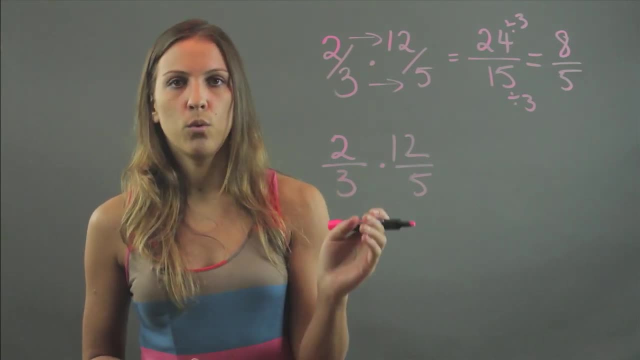 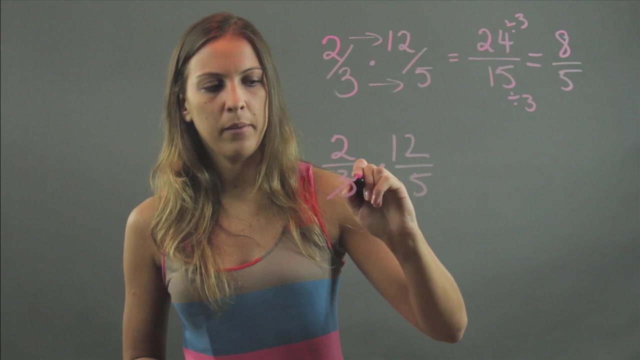 if either of the denominators can be divided into one of the numerators. So 3 can't go into 2, but 3 can go into 12.. So what you do is you cross out the 3, and you say it goes into 12 four times and you replace that 12 with a 4.. 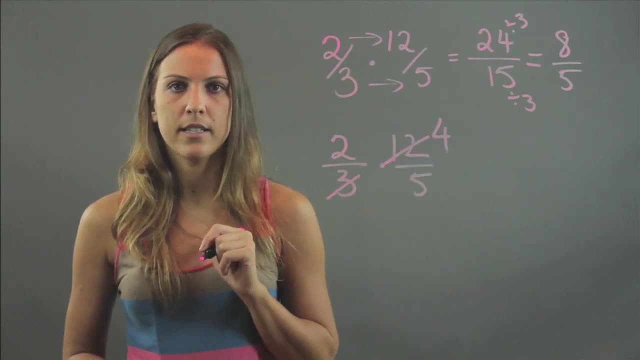 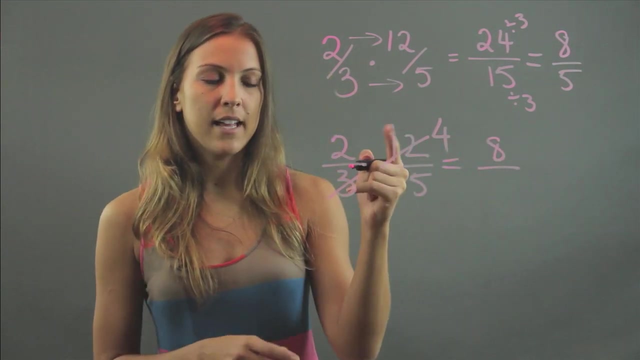 So all I did was 3 goes into 12 four times and I replaced it with a 4.. And now I'm going to go ahead and multiply straight across. so 2 times 4 is 8.. This 3,, when I cancelled it out, actually became a 1, right. 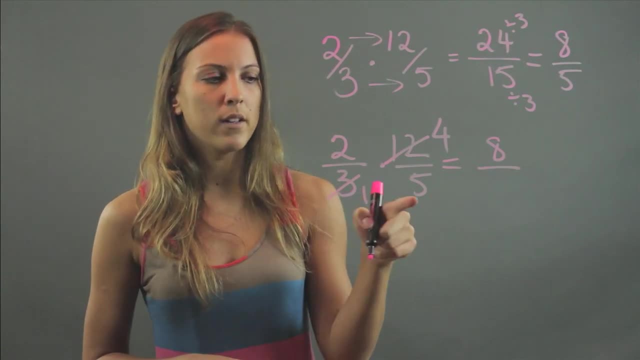 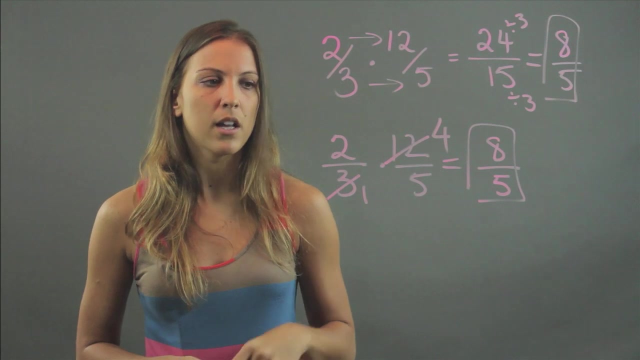 Because what I did was divide by 3, and 3 divided by 3 is 1.. 1 times 5 is 5.. Now I've arrived at the same exact product that I got before. I just did it in a lot simpler fashion. 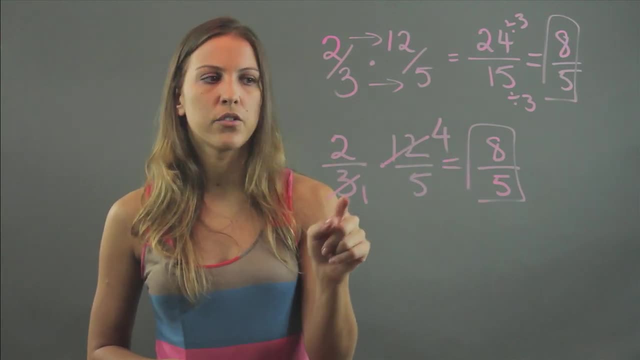 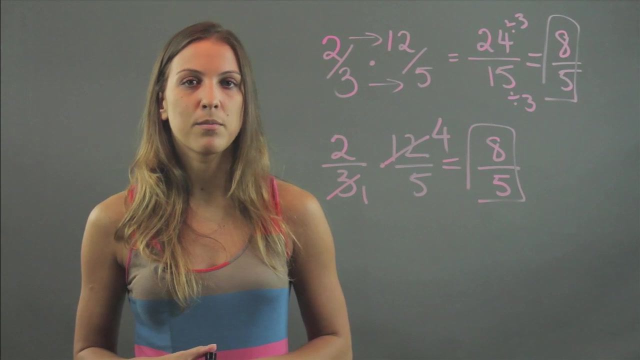 So when you're multiplying fractions, if you see that one of the denominators goes into the numerator, simplify it first and it'll make it easier for you to multiply later. My name is Maria and I just showed you different ways to multiply fractions. 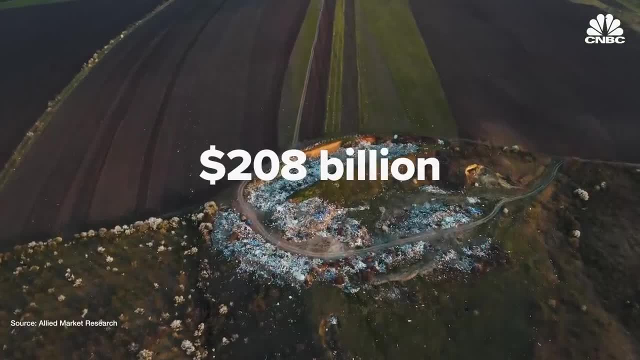 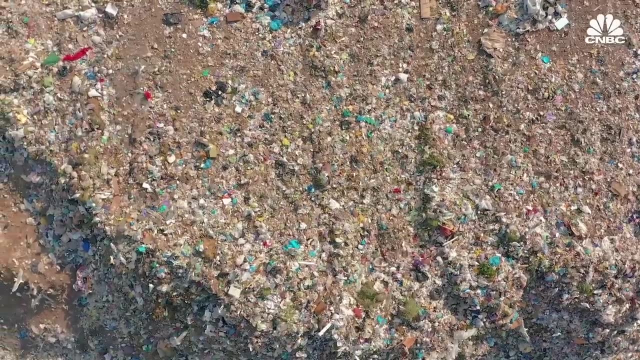 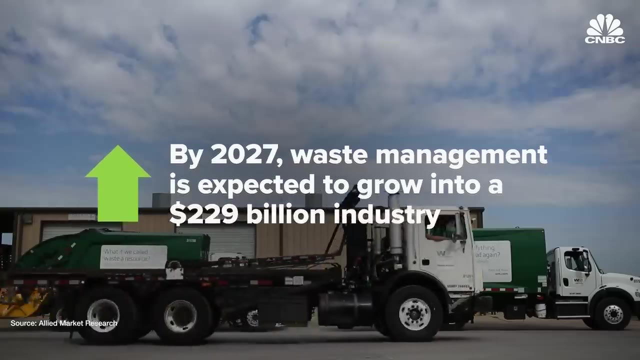 In 2019, the North American waste management market reached $208 billion. Strict environmental regulations, as well as a surge in the amount of waste produced, is expected to expand the market even further. By 2027,, the waste management market is expected to grow into a $229 billion industry.